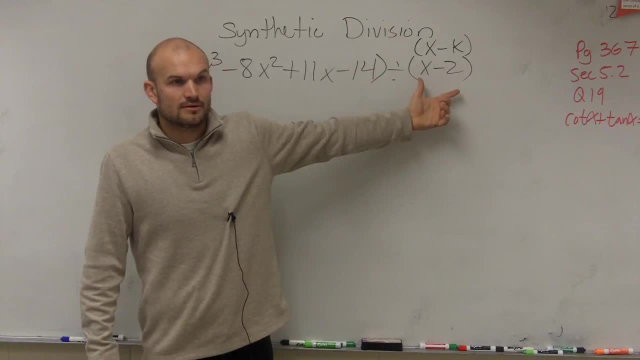 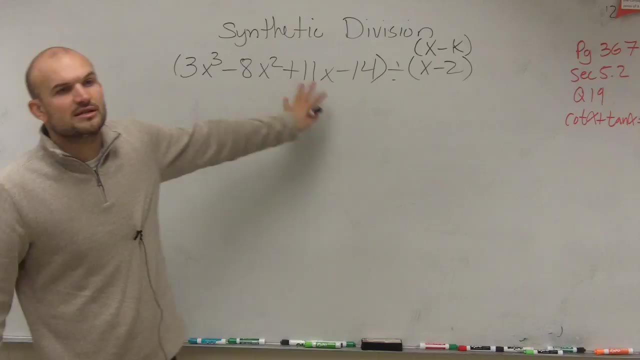 be a factor, It has to be a binomial, linear factor: x plus 2,, 2x minus 1, binomial factor Because if it was just 2x, we'd use the monomial division that we did for number 5.. We use 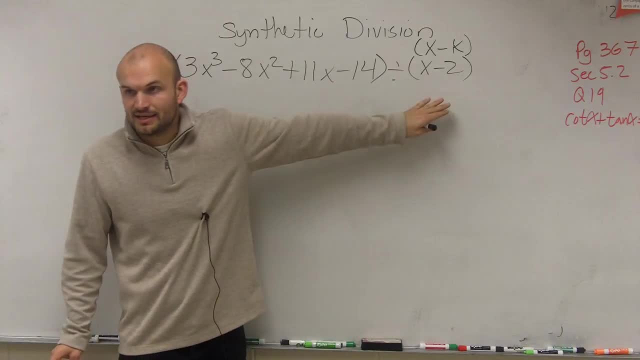 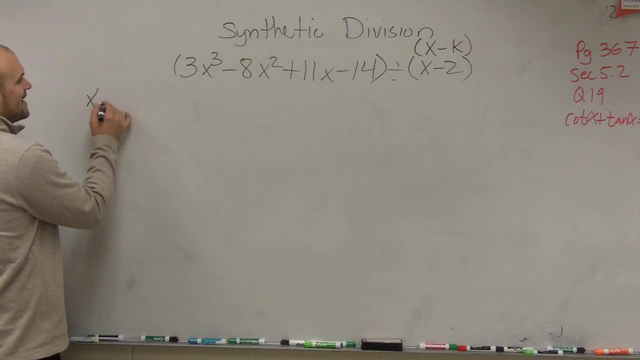 that method. In synthetic division, the main important thing is that you have it as a binomial factor. What you're going to do to figure out, you're going to take your binomial factor x minus k and set it equal to 0.. We'll just start with that for right now. If I do x minus, 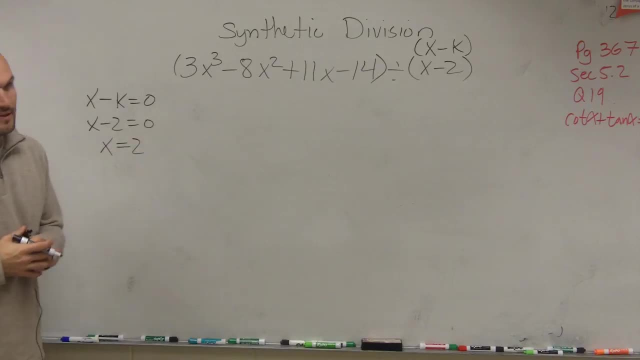 2 equals 0, I'm going to say x equals 2.. That's going to be our version of k, which we're going to write. We're going to write 2 on the outside. We're going to make a little L-shaped box Like 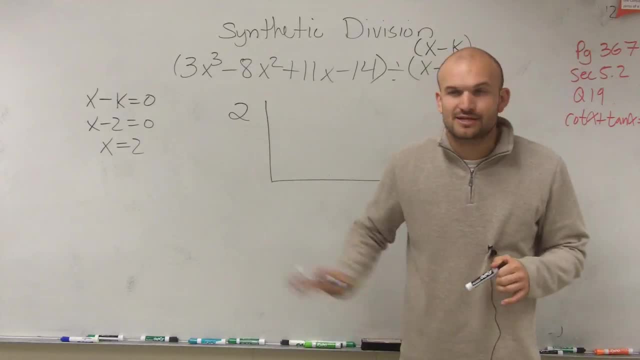 I said right now I'm not going to get deep into the synthetic division, why we do this. I just want you guys to write down the process and follow along. Once we talk more about zeros and stuff like that, we'll learn more how synthetic division is going to help us. 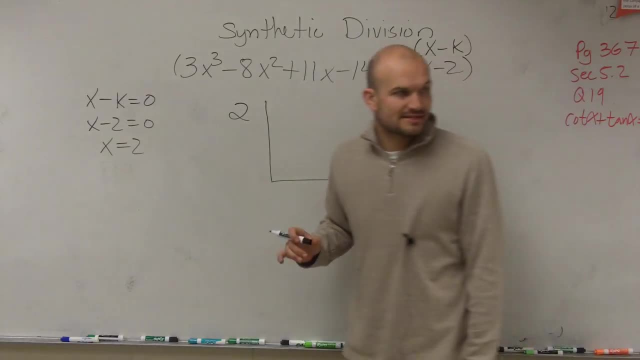 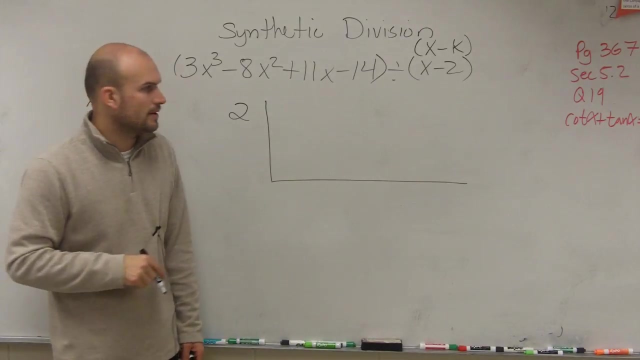 out. Right now we're just learning the process. I'll explain a lot more why we're going to do and how we're going to do things in a second. I just want you guys to be writing down the process Now. what we're going to do is we're going to take each coefficient of our terms and 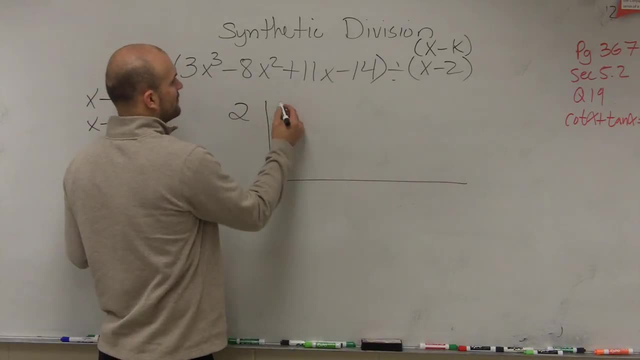 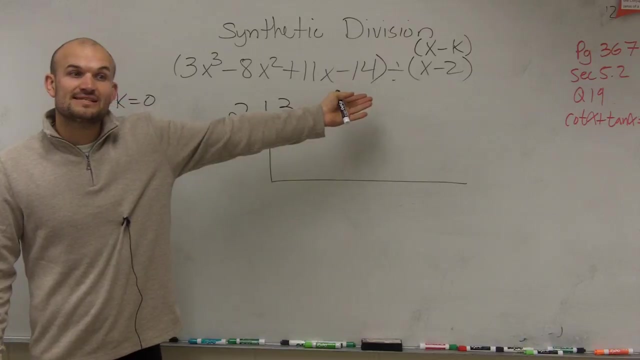 write them in an invisible column. Our first term, our first coefficient, is 3.. We're always going to start with the leading term and make sure you go in descending order. If you are missing a term, like say, there was no 11x, then you'd put a 0 there Or, sorry, a 0x. 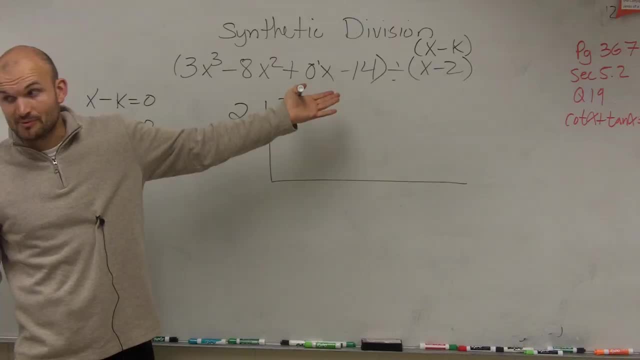 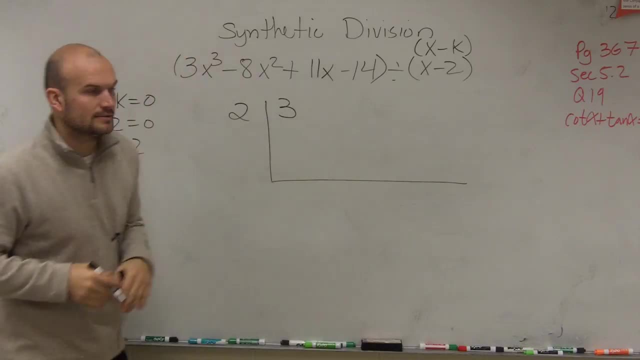 Now, what else do you want us to do? All you want to do is take the negative 10 to the highest of the minus 1.. So you can do a third term And you can do a third term, But if you do have an x, we have an 11x. All I'm saying is you do 3, negative, 8,, 11, and negative. 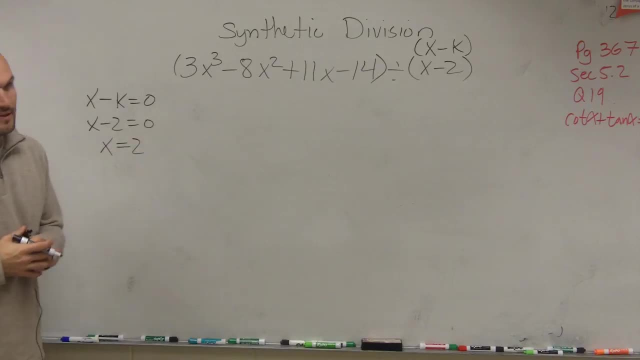 2 equals 0, I'm going to say x equals 2.. That's going to be our version of k, which we're going to write. We're going to write 2 on the outside. We're going to make a little L-shaped box Like 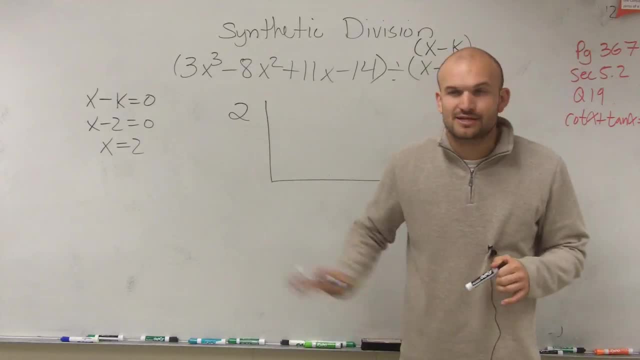 I said right now I'm not going to get deep into the synthetic division, why we do this. I just want you guys to write down the process and follow along. Once we talk more about zeros and stuff like that, we'll learn more how synthetic division is going to help us. 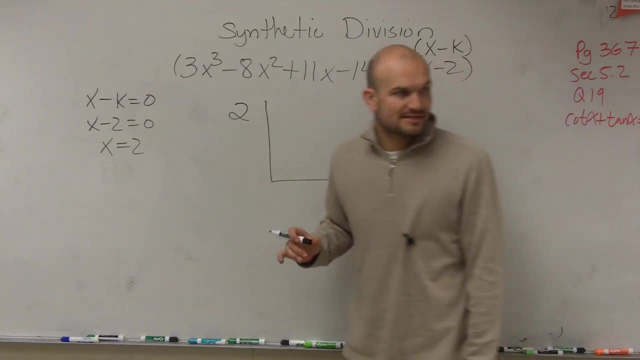 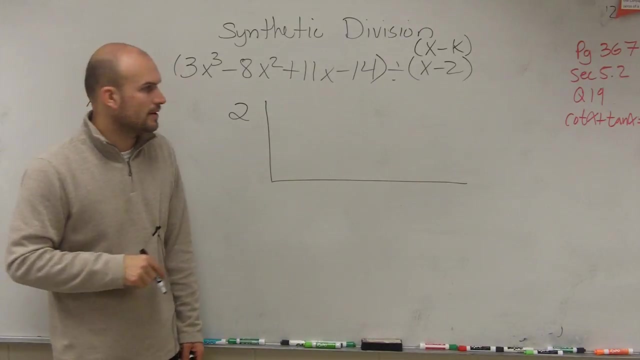 out. Right now we're just learning the process. I'll explain a lot more why we're going to do and how we're going to do things in a second. I just want you guys to be writing down the process. So what's going to do is we're going to take each coefficient of our terms and write. 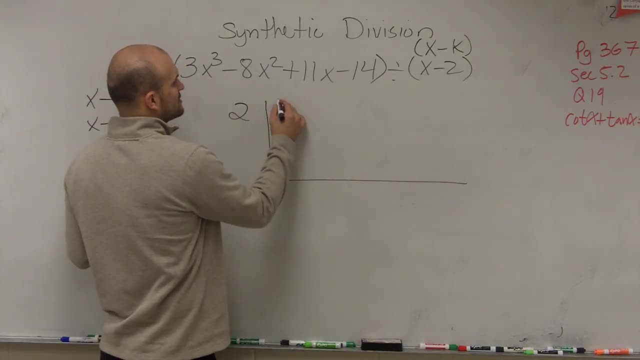 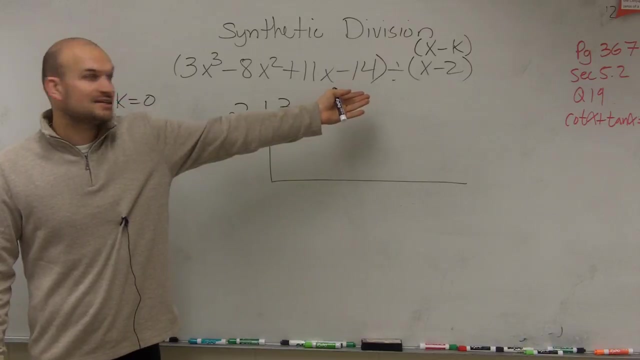 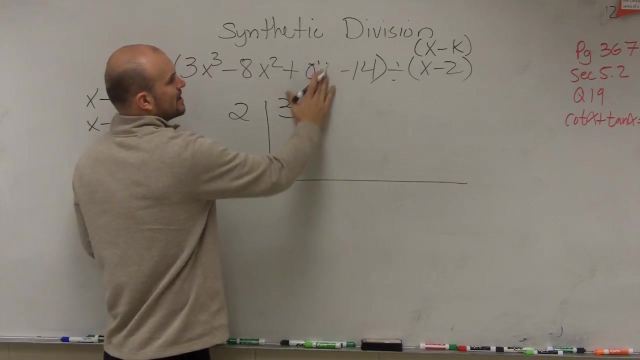 them in invisible column. So our first term, or first coefficient's three, We're always going to start with the leading term and make sure you go in descending order. If you are missing a term like, say, there was no 11x, then you'd put a zero there. Sorry, zero. 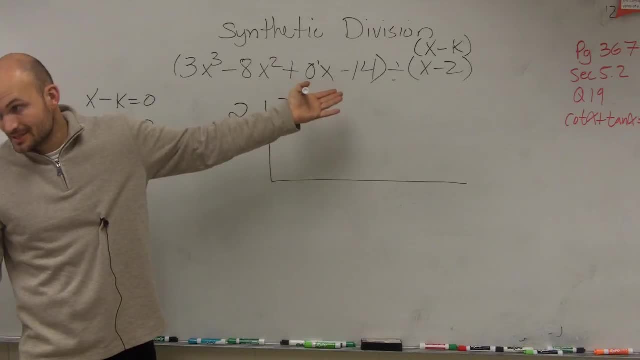 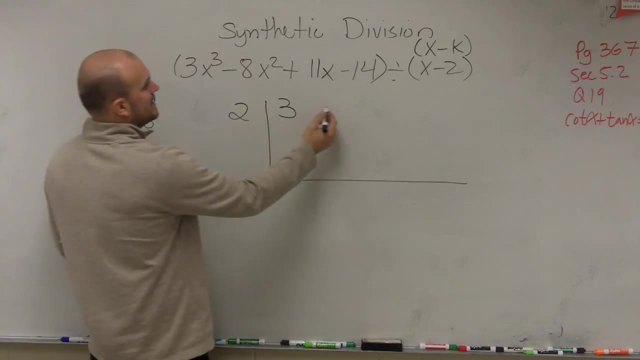 x. If there is no term there, you would put a 0. But we do have an x, We have an 11x. All right, All I'm saying is: so you do 3, negative 8,, 11, and negative 14.. So you take. 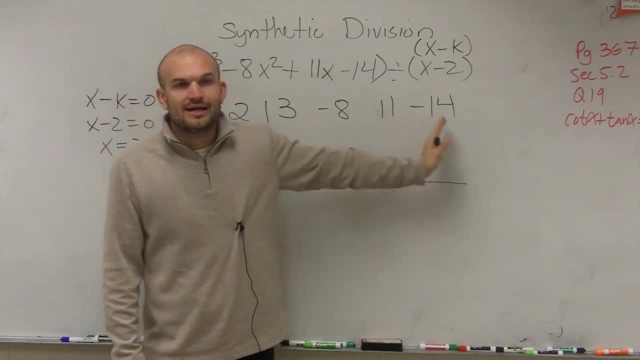 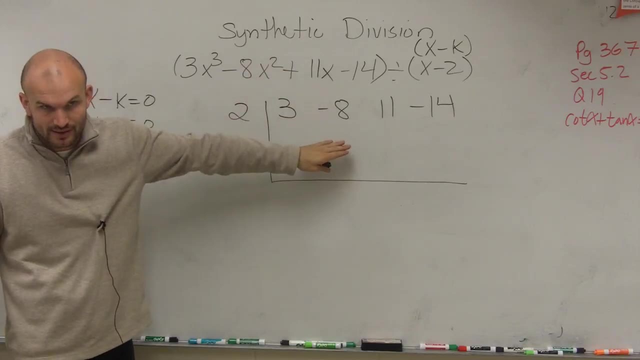 all the coefficients and the constant and you make sure you list them in their descending order from their polynomial. All right, If you did not have a term you would put a 0 in there, Just saying you have to make sure you include every single degree from descending. 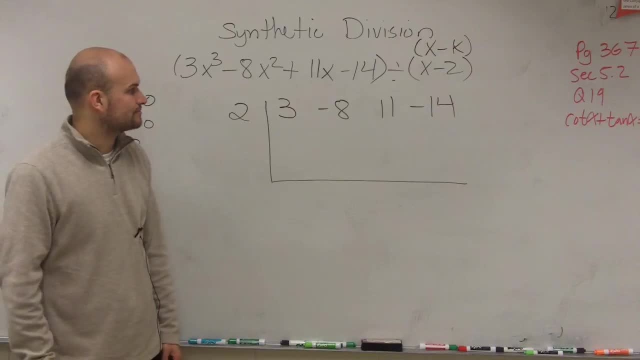 order. Okay, We'll do a problem where we're missing one. All right, So now the synthetic division algorithm goes like this: The first number we like to sometimes say it's a freebie, So you just bring it directly down, So we get 3.. Then what we do is: you do 3 times 2.. 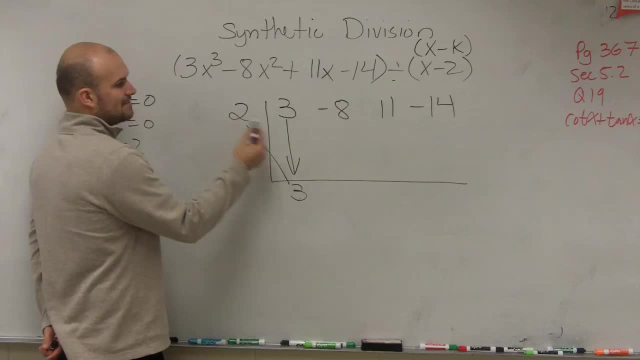 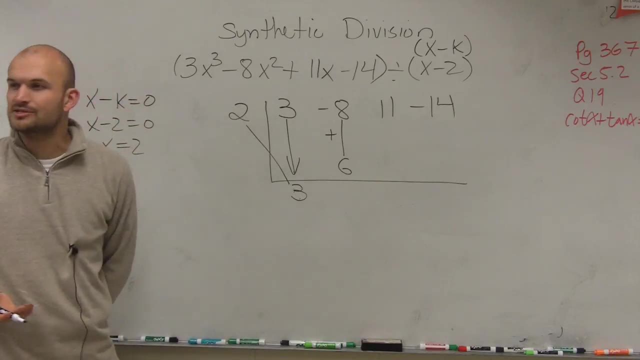 So the diagonals you multiply 3 times 2.. 3 times 2 is 6.. Then we vertically add. And this is why a lot of people like synthetic division because there's no, we're not subtracting anymore, We're adding. So negative, well, adding. 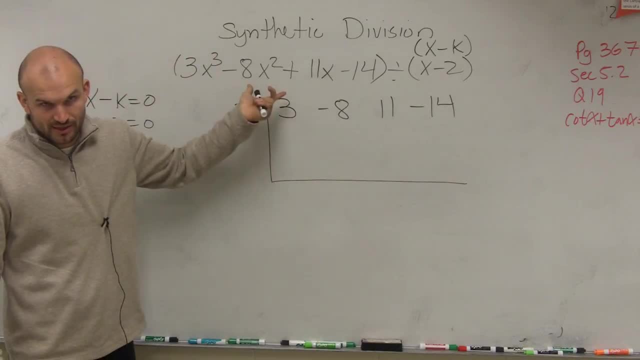 14. So you take all the coefficients and the constant and you make sure you list them in their descending order from their polynomial. If you did not have a term you would put a 0 in there, Just saying you have to make sure you include every single degree from descending order. 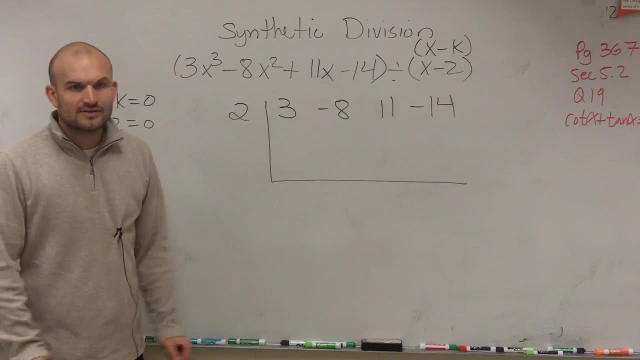 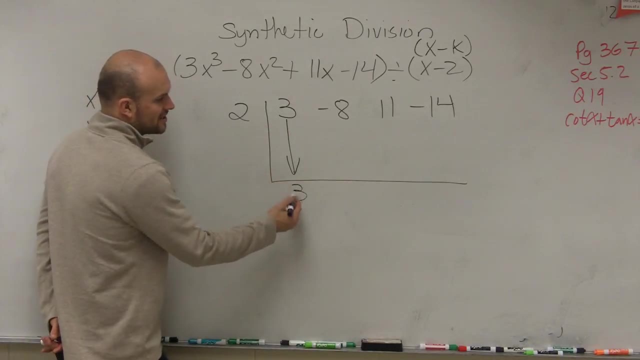 Okay, one, Alright. so now the synthetic division algorithm goes like this: The first number we like to sometimes say it's a freebie, so you just bring it directly down, So we get 3.. Then what we do is: you do 3. 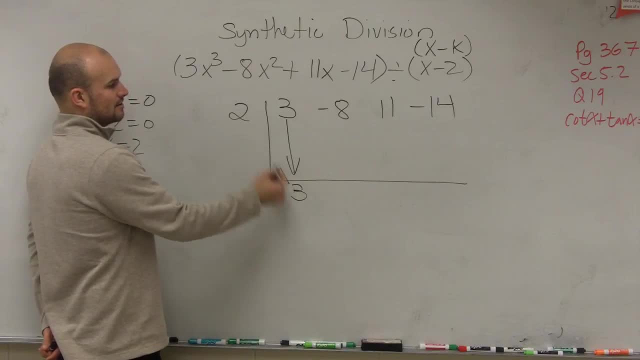 times 2.. So the diagonals you multiply 3 times 2 is 6.. Then we vertically add, And this is why a lot of people like synthetic division, because there's no, we're not subtracting anymore, we're adding, So negative. 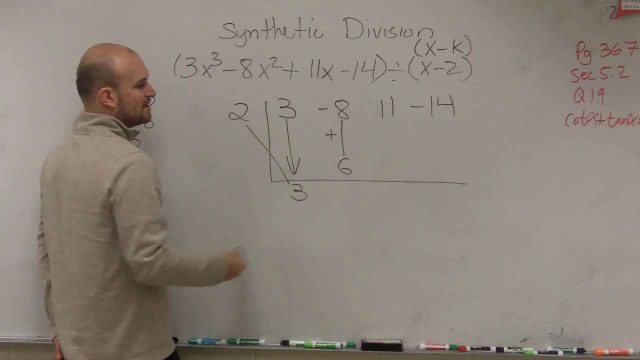 well, adding the negative is kind of saying we're subtracting. but negative 8 plus 6 is negative, 2. Then multiply the diagonal Negative 2 times 2 is negative, 4.. Add 11 plus negative: 4 is positive, 7.. 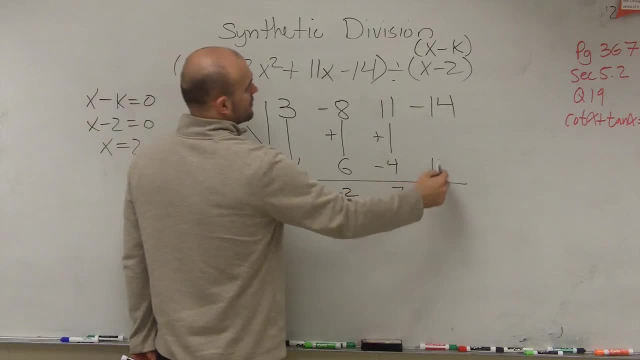 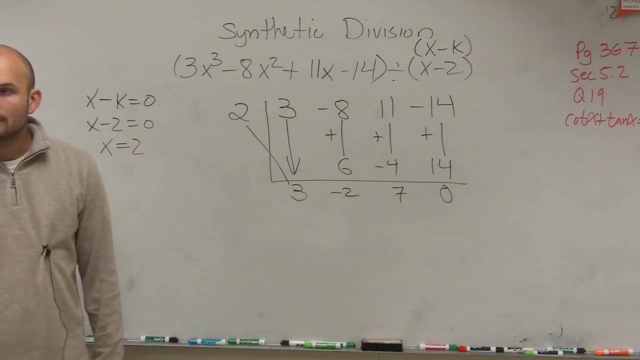 Multiply the diagonal 7 times 2 is 14.. Add the vertical: 0.. Now we write our answer. The first answer or the last answer we have is always our remainder. In this case, we have a remainder of 0.. The next case is our constant. 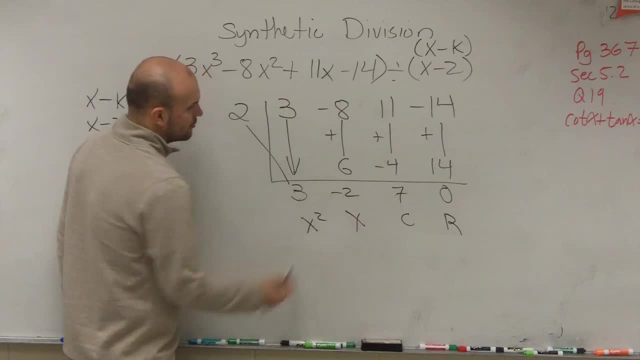 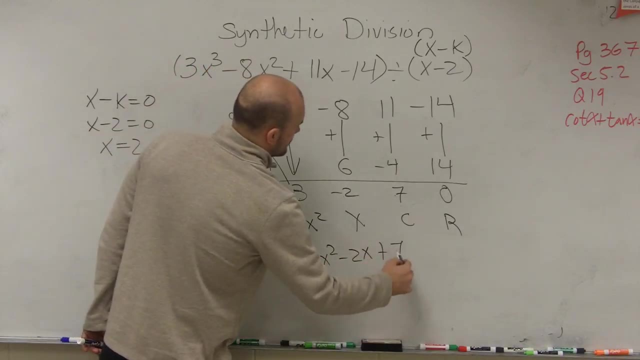 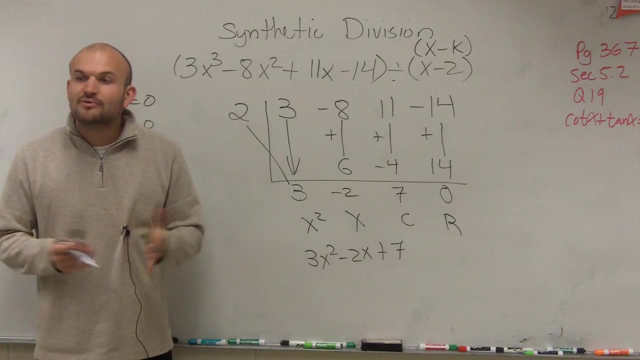 Then we have our linear and then we have our quadratic. So our final answer is 3x squared minus 2x plus 7.. Cool, Pretty easy, right, Remember? it's pretty basic compared to our long division method. The difference is, ladies and gentlemen, 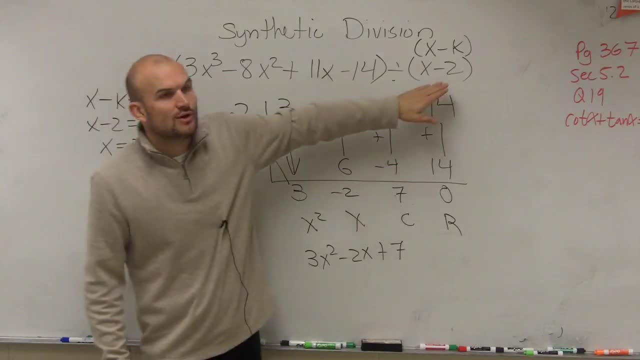 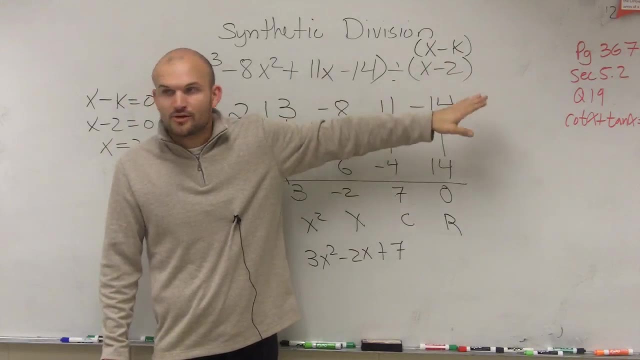 you have to. you can only use this when you are dividing by your x minus k, When it's in that format, When you can write it as a linear binomial. If it's not as a linear binomial, we cannot apply synthetic division. So it's very important for you guys to know long. and synthetic: Yes,